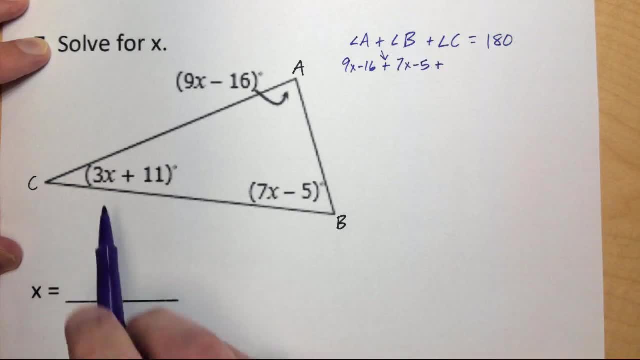 angle B Bring down our other plus sign, And for C we know that as 3x plus 11. And all of that added together is going to equal 180.. Now we can combine the things that we know here. We have a bunch of x's and we have 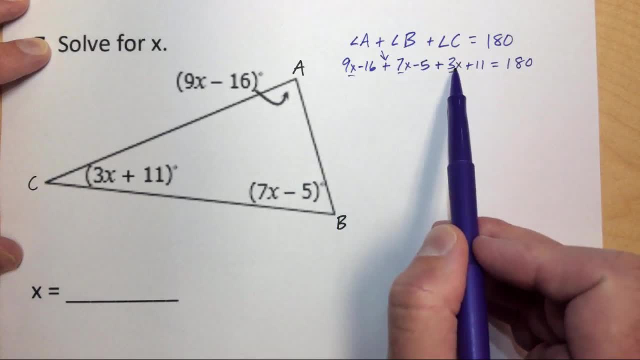 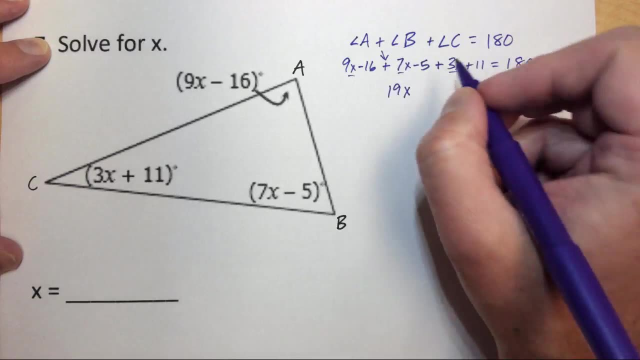 a bunch of numbers And if we combine all of our x values, we have 3x's here, 7x's here and 9x's here. Add those all together we have 19 total x values. So we have 19x. We've. 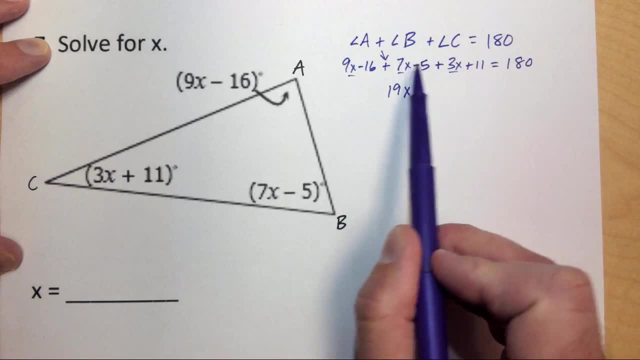 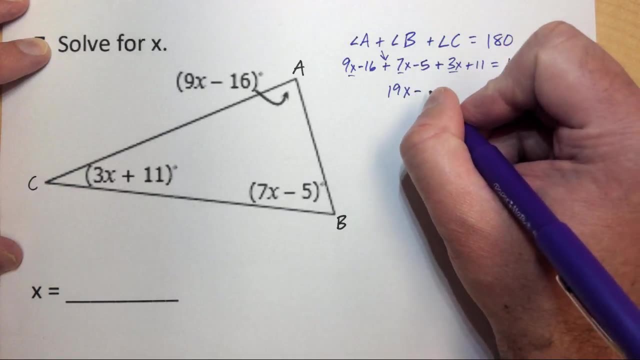 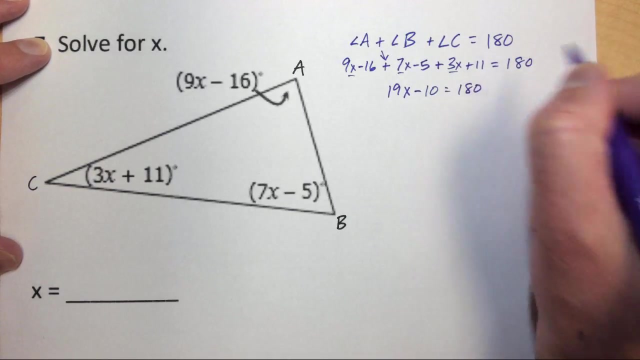 subtracted 16, subtracted 5, and then added 11.. If we combine these, we're subtracting 21 all together. Subtracting 21 to add 11, we still are in the negative, but we end up subtracting 10 once we combine all those numbers And again all that equals 180 degrees Add. 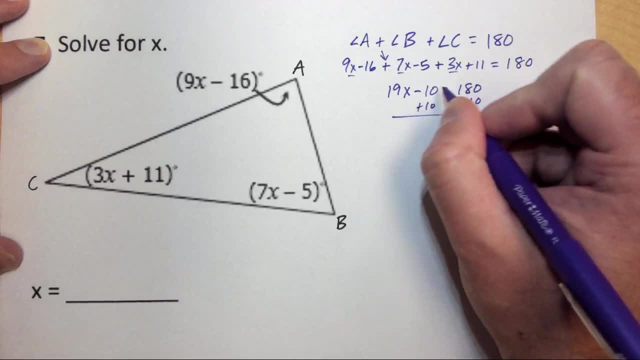 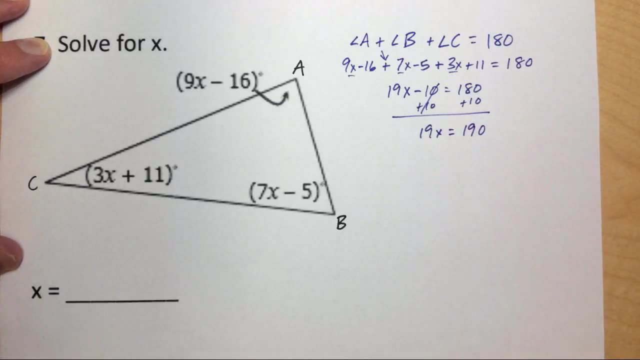 10 to both sides, We end up with 19x on the left-hand side of our equation, 190 on the right-hand side of our equation. now that we've got our x values all by themselves over here, Divide by the multiplier of 19 on both sides and we'll find that x is equal to 10.. Now we can use: 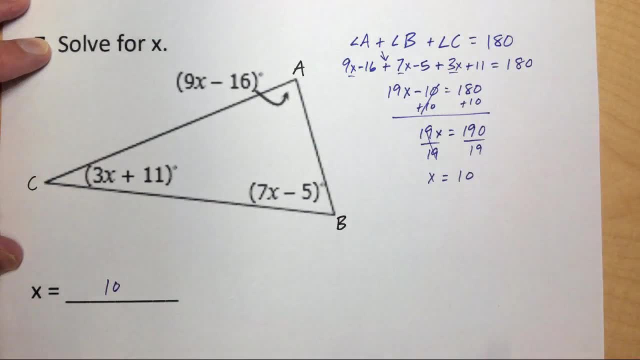 that and we can plug that in. That's our answer for our problem. but let's just double check to make sure everything works by plugging it into each particular equation. So where we see x, we're going to plug in 10. We're going to substitute that 10.. So 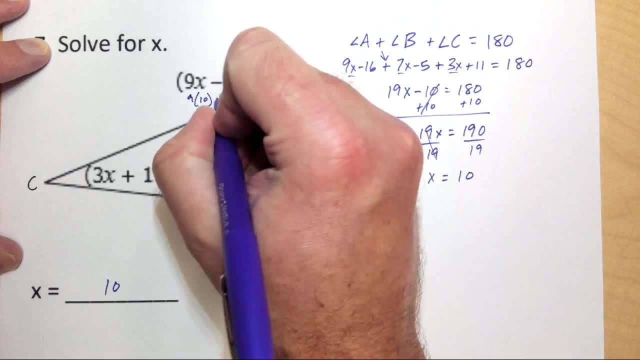 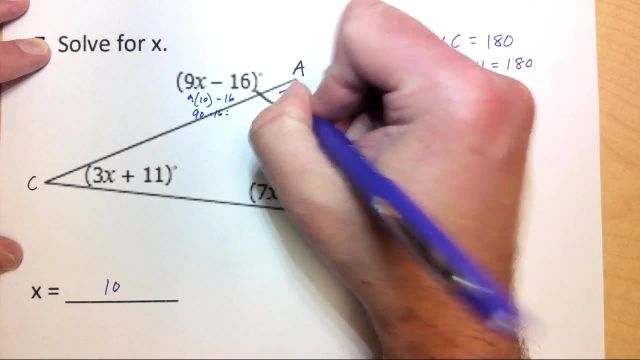 for angle A, for instance, we have 9 times 10 minus 16.. 9 times 10 is 90. Minus 16 gives us an angle measurement of 74 degrees. This should be 74 degrees 7 times 10 for angle. 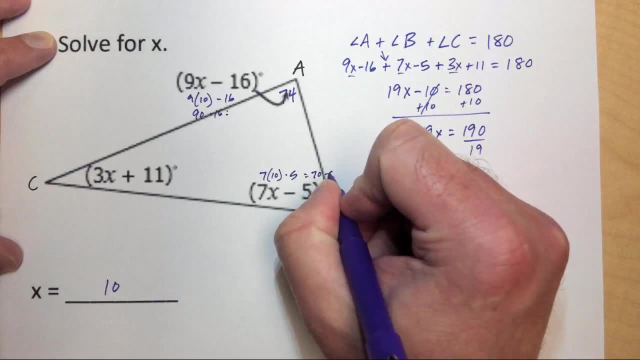 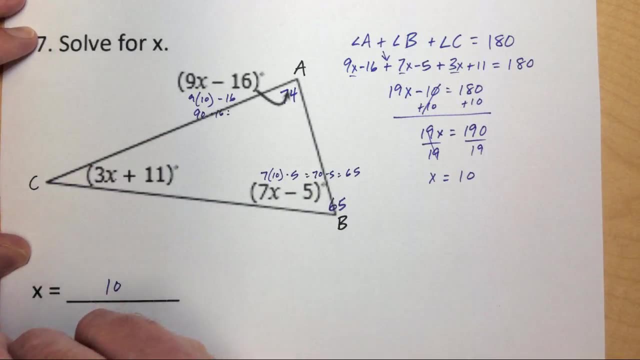 B minus 5 is 70 minus 5, which should be 65 degrees. This should be a measurement of 65 degrees And if we substitute it in for our C, we have 3 times 10 plus 11, which is: 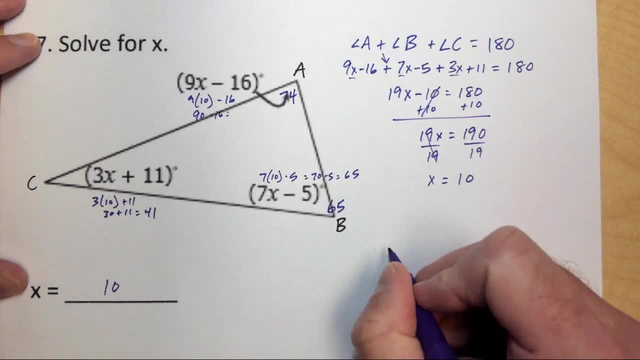 30 plus 11, which is 41 degrees. Now, again, based on our rule that we already know, angle A, which should be 74,, angle B at 65, and angle C at 41 should all add together to equal 180 degrees. And when we do this,